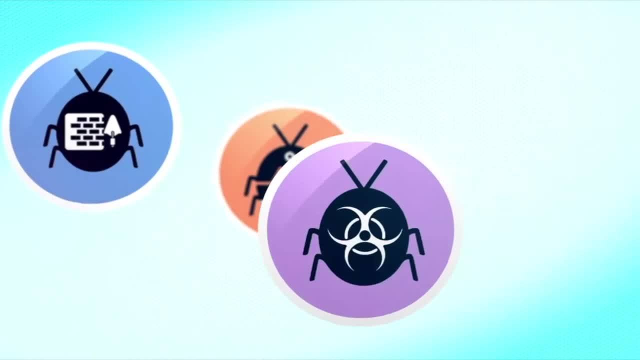 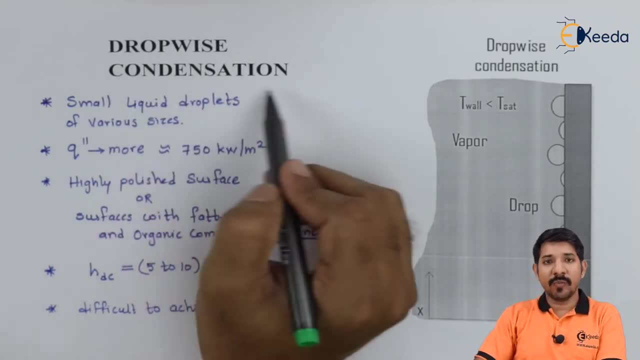 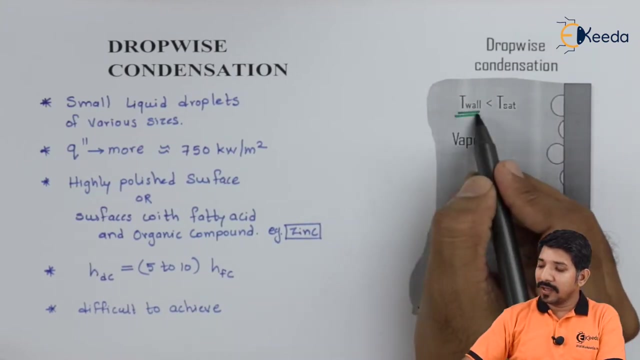 So what do we have in case of a drop wise condensation? Again, consider a small wall whose temperature is, let's say, TW, and we have made sure that the TW is less than the T saturated. Now, what is T saturated? It is the saturation temperature for a given vapor which is there. 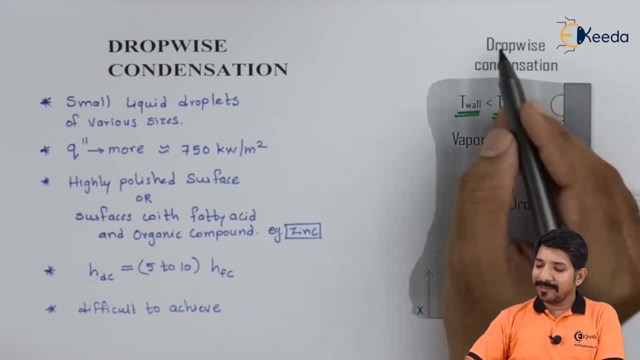 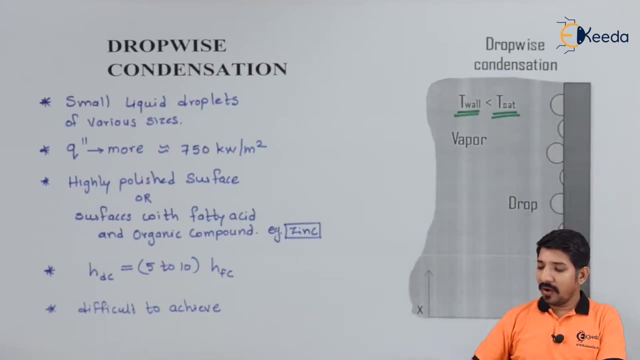 around the wall. So what will happen in case of a dropwise condensation? a small drops will be formed over the wall or over the surface of a given wall. Now these droplets can be of various shape and size. Now, this will depend on so many parameter. the most important parameter will be the 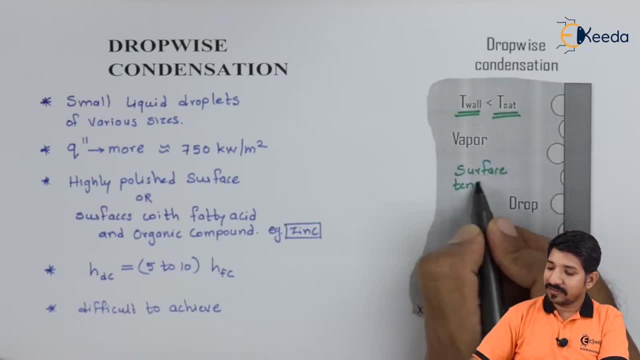 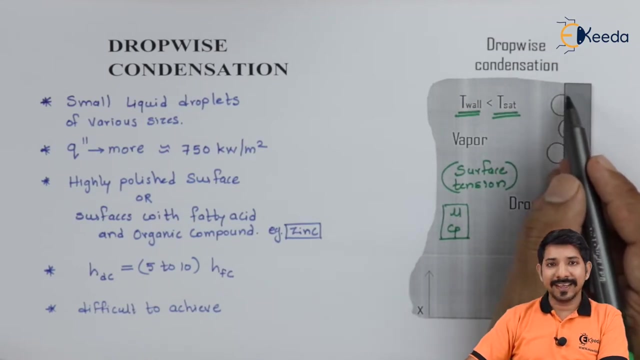 surface tension. Apart from surface tension, it is the mu and Cp value for the given fluid that will decide what should be the size of a bubble that is formed over a wall. So, basically, the important parameter in this case that need to be understand is that in the dropwise 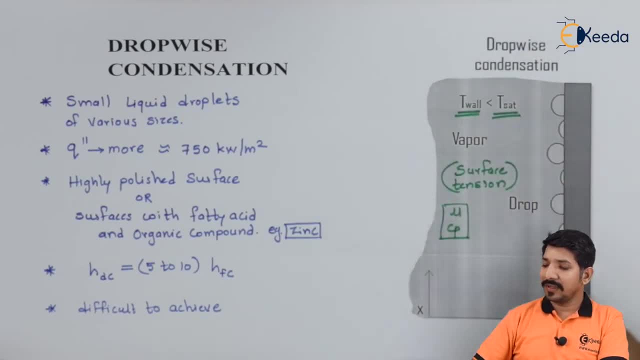 condensation, small bubbles are formed over the wall. So basically the important parameter in this case that need to be understand is that in the dropwise condensation, small bubbles are formed over a surface, So it will never wet the entire surface. Small surface will always. 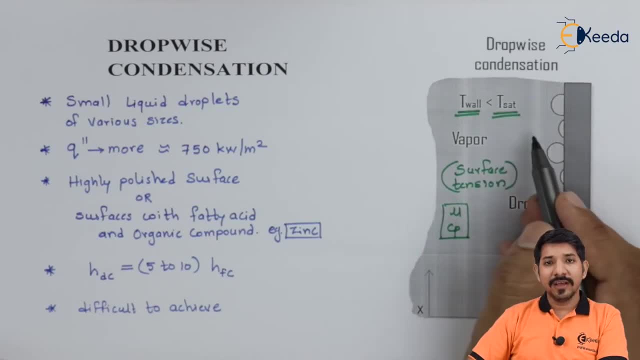 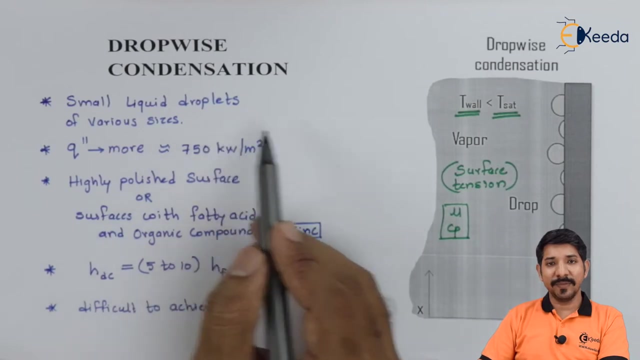 be exposed to the vapor, So that will enhance the heat transfer rate in case of a dropwise condensation. So these are some of the silent feature which I have written down here. In case of a dropwise condensation, a small liquid droplets of various size and shape will be. 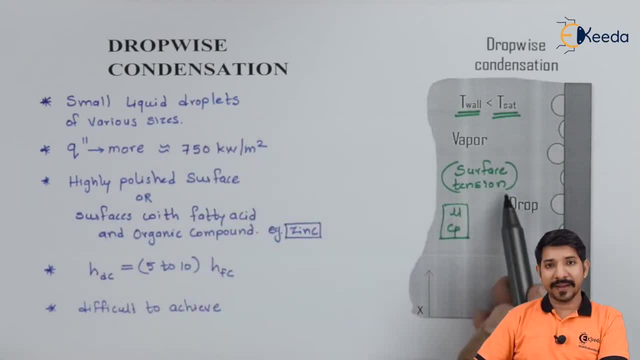 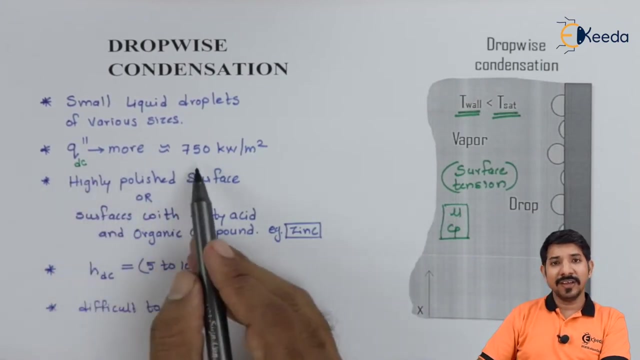 formed. The size and shape may depend on these many parameters. The heat transfer rate or the heat flux are more as compared to that of the film wise condensation. So for dropwise condensation the heat flux is more than that of the film condensation. to what amount? So? it is estimated that approximately 0.75 megawatt per meter. 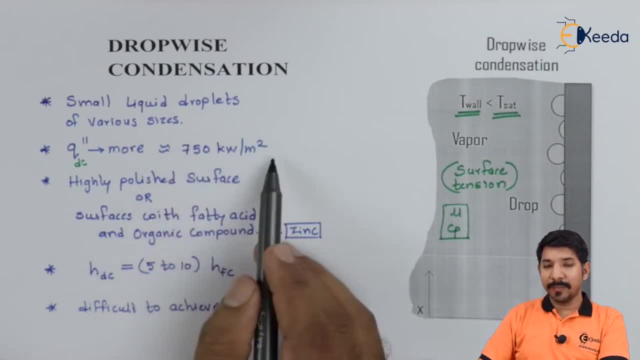 square or 750 kilowatt per meter square is the amount by which it is more than that of the film wise condensation. Similarly, we can say that the heat transfer coefficient in case of a dropwise condensation is 10 to 5 to 10 times more than that of the film condensation. So what decides if the condensation? 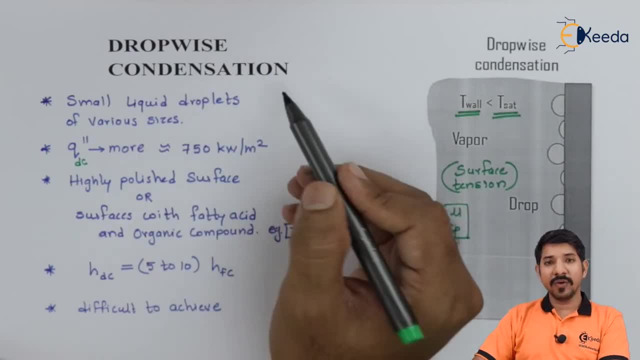 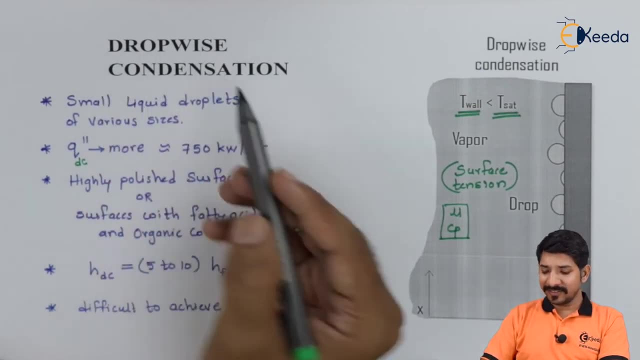 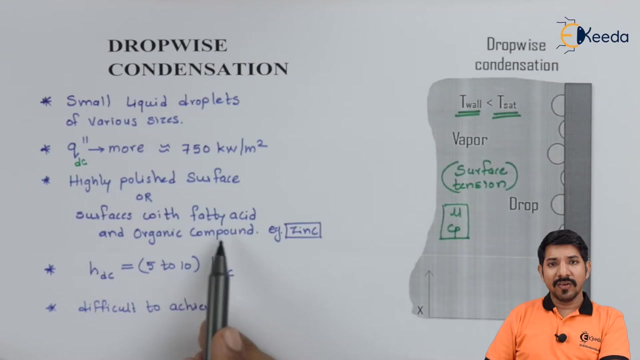 is a dropwise or film wise. So that will be depending on the surface. If the surface is highly polished, then we will obviously end up getting the dropwise condensation. or if the surface is there with the fatty acids Or organic acids or organic compound, then we are going to get a dropwise condensation. 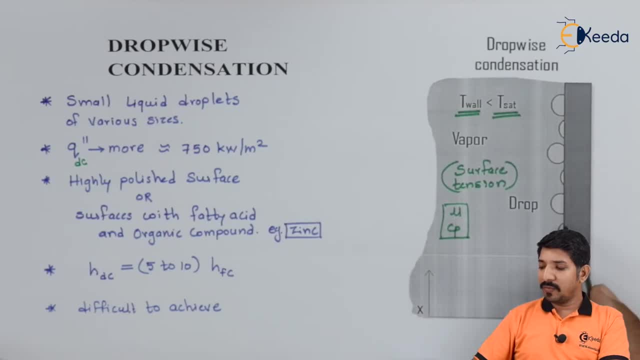 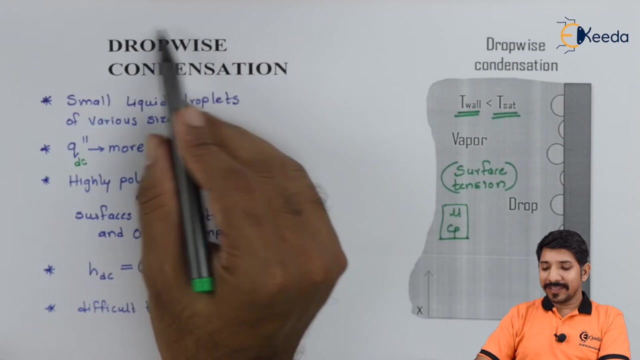 So if we take a, let's say, a small fatty acid compound, if we apply it onto the surface of a given wall, then we are going to end up into the dropwise condensation itself. The only point with the dropwise condensation is that it is quite tough to achieve, because 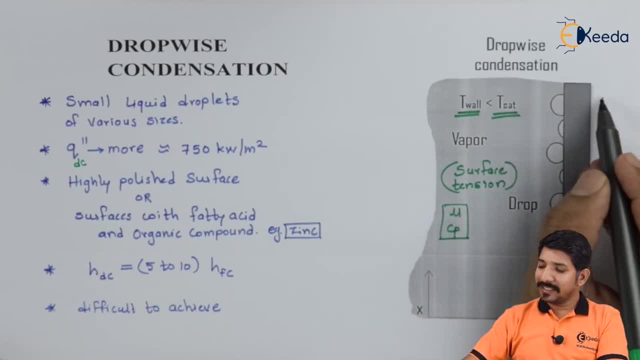 of the gravity. So in the first of the scenario, what will happen? due to the gravity, this drop will start falling and then a small film will be formed over a surface. But this is a gradual activity, but initially, when the time is less, if we get a small droplets onto the surface, 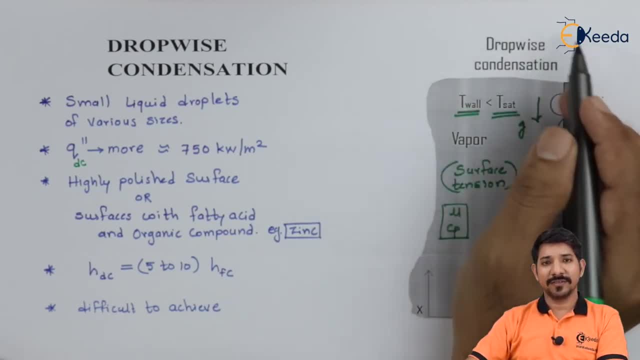 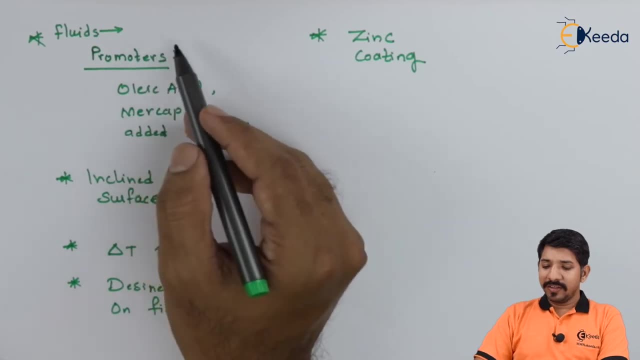 then that kind of condensation is a dropwise condensation. Now here I have listed some of the things that we can do to enhance the condensation, So let's see what happens. The first thing is we can obviously coat the given surface with the zinc. We can either: 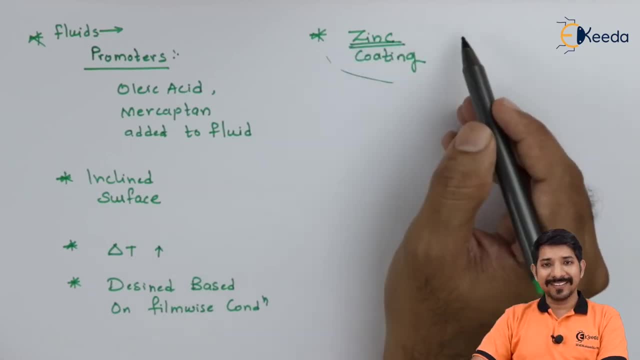 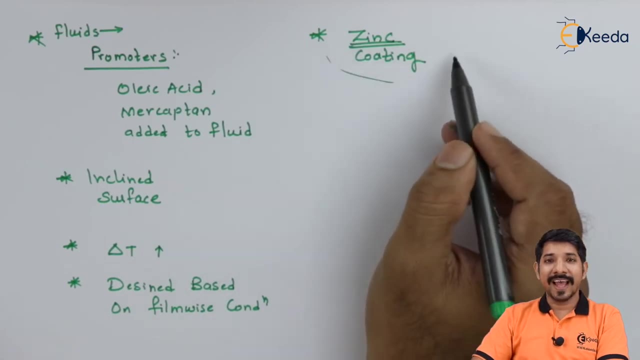 coat it with the zinc or any other fatty acids. that will enhance the dropwise condensation. or we can even make the surface highly smooth, so that will also enhance the dropwise condensation. So this is what we can do about the surface. We can also add some of the content to the 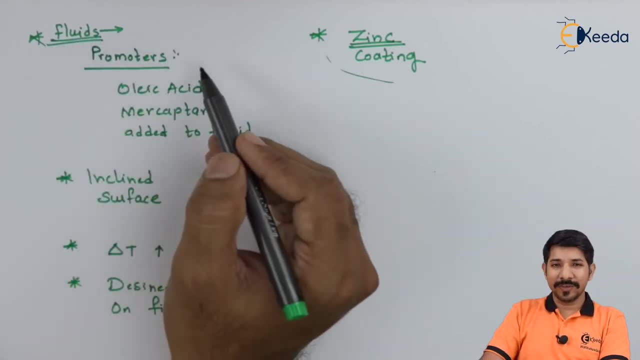 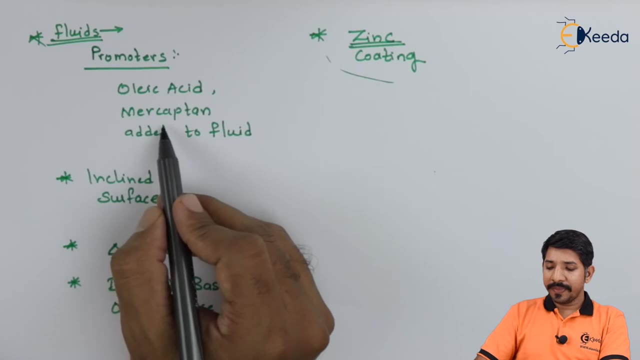 surface. So this is what we can do about the surface. We can also add some of the content to the surface. We can also add some of the contents to the fluid that will enhance the dropwise condensation. So those contents they call as the promoter. 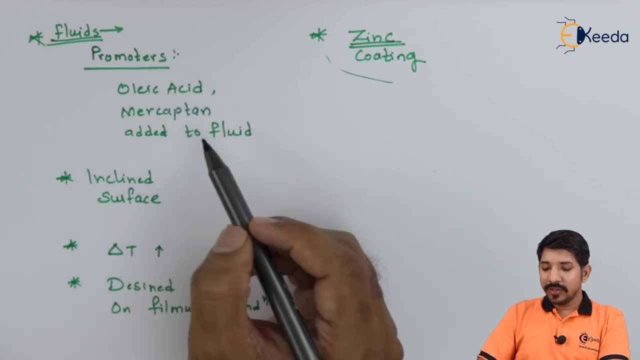 those are nothing but oliva acid or Markeptin. one 이런 점을 poner 주 할 때 gibi Ora ekiam. Things are little compounds that is added to the given fluid to enhance the dropwise condensation. One more thing that we can do. 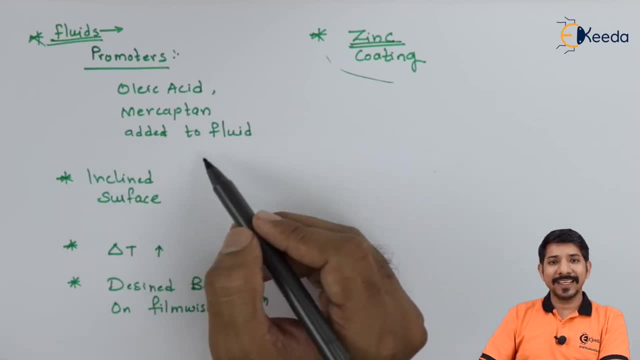 one more thing that we can do to enhance the heat transfer rate in case of condensation is by making the surface inclined. See, if I make the surface inclined, what is going to happen? whatever the film or the drop that are formed onto the surface, those will obviously get. 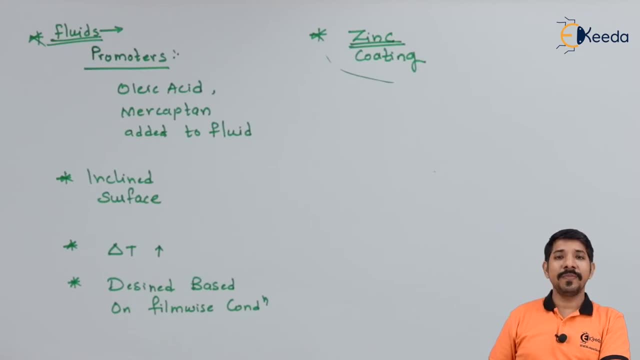 eliminated or those will obviously come down and that will expose the surface to the vapor and that will obviously increase the heat transfer. to make the delta T high: if I make the delta T high, that is if I make sure that T wall minus T sat is quite high now in that 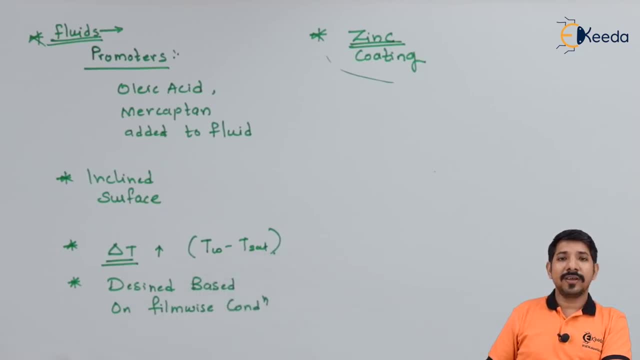 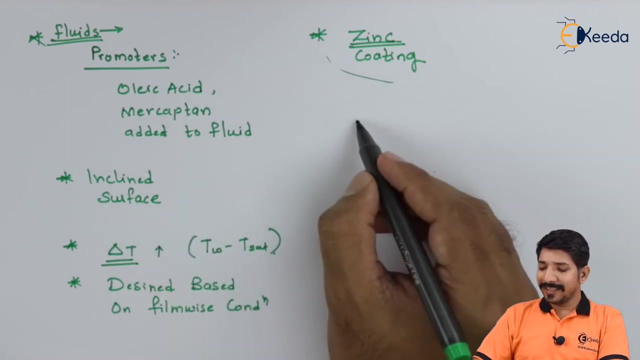 case, what is going to happen? obviously, the condensation will be fast in this case, and then, due to the higher mass flow rate, the surface will get vacated quickly and in turn, that will increase the heat transfer rate. now, by saying all these things to improve the heat transfer rate, one can obviously understand that if we try to achieve a drop something, 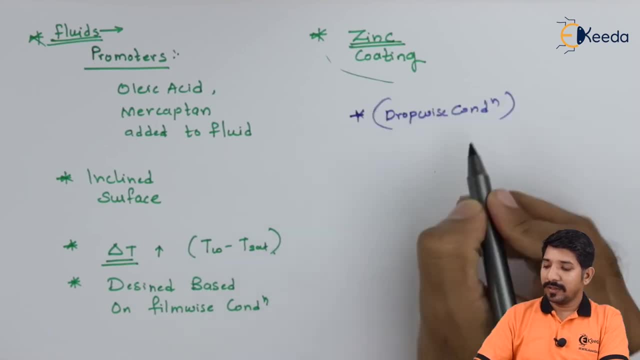 like this right. so whatever it is, if B II is acting like in that case, B II is acting like in that case. so whatever it is, if B II is acting like in that case, so whatever it, drop wise condensation, then the value of heat transfer rate is quite high. but there is a 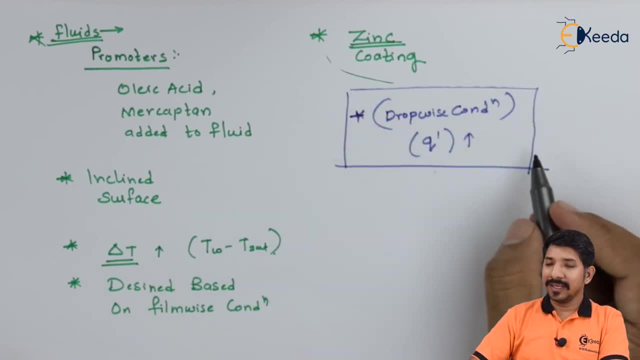 problem in achieving drop wise condensation. practically speaking, it is not that easy to achieve the drop wise condensation. in most of the scenario, we will always end up in getting the film wise condensation now. that is why it is always recommended to design any given condenser. we always have to imagine, or the design has to be based on, the film wise condensation. 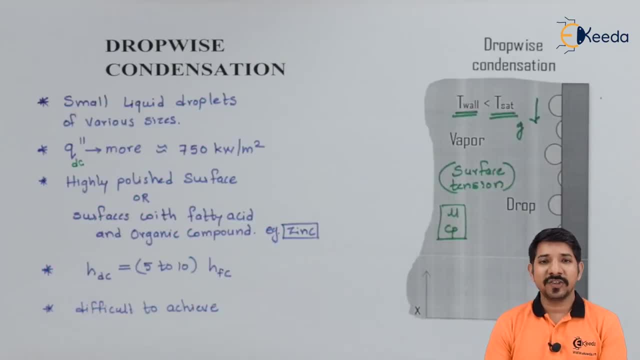 only now. that is it in this topic. in this topic, we talked about what do you mean by the drop condensation and its comparison with the film wise condensation. we have also talked about various methods by which how can we increase the heat transfer rate in case of a condensation. 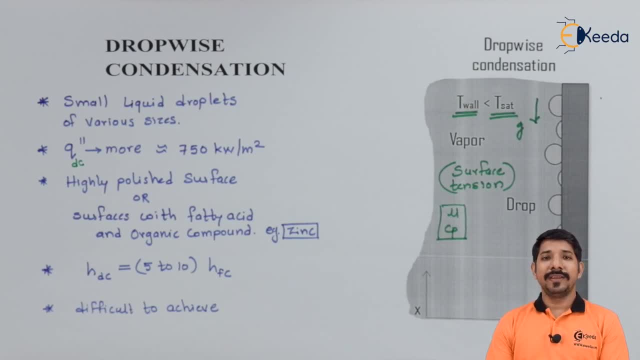 now, that is it in this topic. thank you for watching this video. please stay tuned with me and i will see you in the next video, VIKIDA, and subscribe to VIKIDA, Thank you.